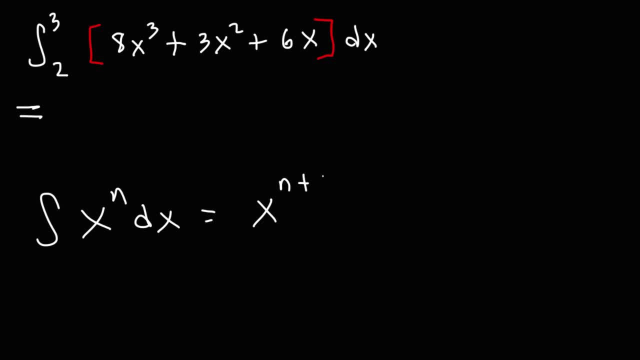 going to equal that variable raised to the constant plus 1, divided by n plus 1.. Now for indefinite integrals. we would have the constant of integration, c. But when dealing with definite integrals, you don't need to worry about c. 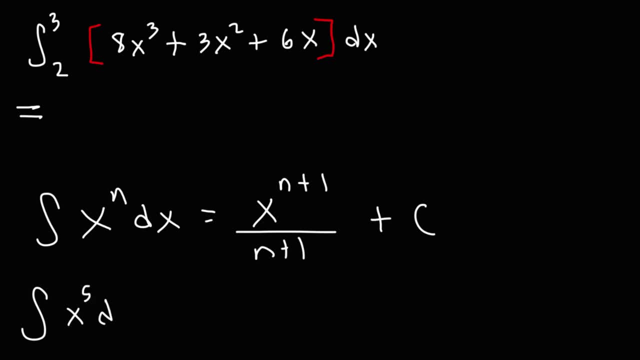 So, as an example, let's say, if we want to find the antiderivative of x to the fifth, all you need to do is add 1 to the exponent- It's going to be x to the sixth- and then divide by that result. 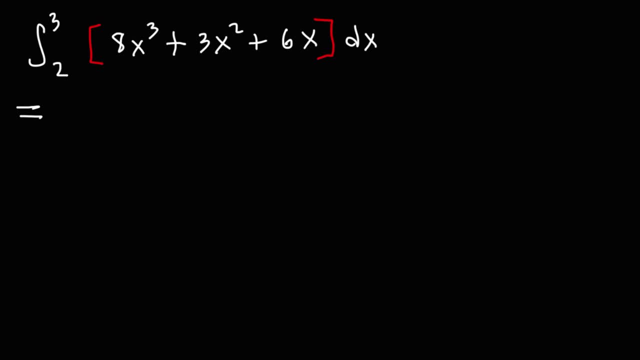 So let's say, if we want to determine the antiderivative of 4x to the seventh- So we have a constant times x to the seventh- First rewrite the constant and then find the antiderivative of x to the seventh. 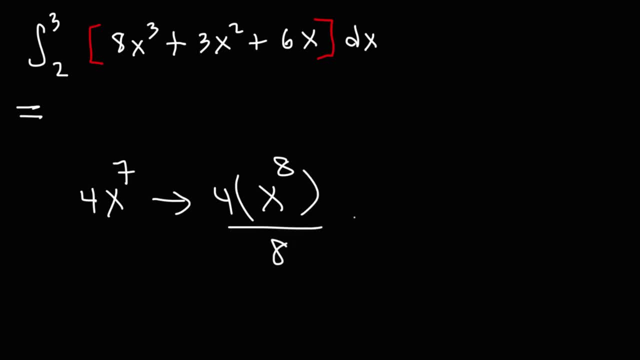 So add 1 to 7, that's 8, and then divide by that number, And after that you can reduce it. So 8 is 4 times 2.. We can cancel the 4, and so the answer is going to be x to the 8 over 2.. 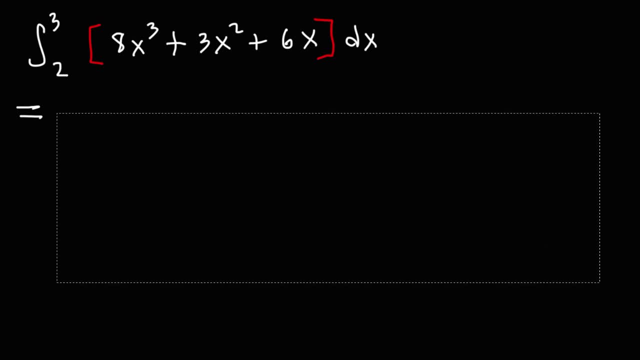 So that's how you could find the antiderivative of monomials. Now let's continue on with this example. So to find the antiderivative of 8x cubed, first we're going to rewrite the constant 8.. 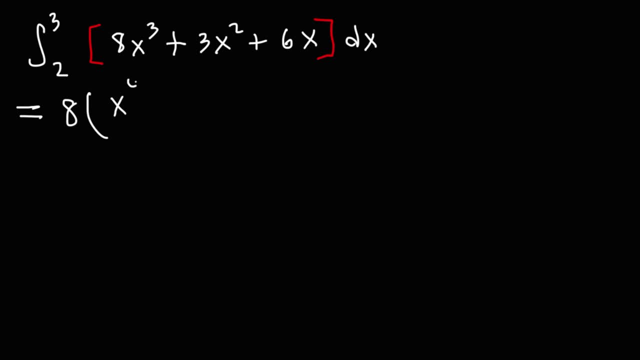 Then we're going to add 1 to the exponent. 3 plus 1 is 4.. And then we're going to divide by 4.. Now let's repeat this process for the next one. So the antiderivative of 3x squared is going to be the constant 3 times x raised to the third power, divided by 3.. 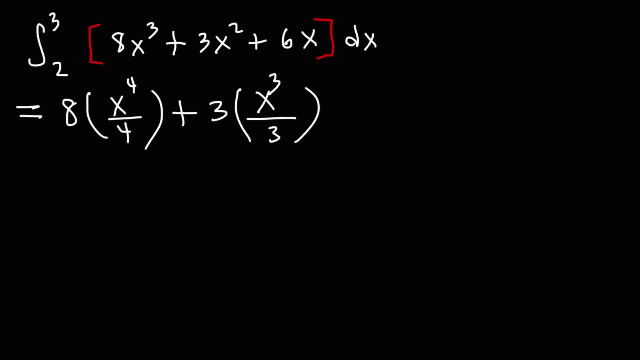 Now, what about the antiderivative of 6 times x? If you don't see a number, it's always a 1.. This is 6 times x to the first power. So, just like before, we're going to rewrite the constant. 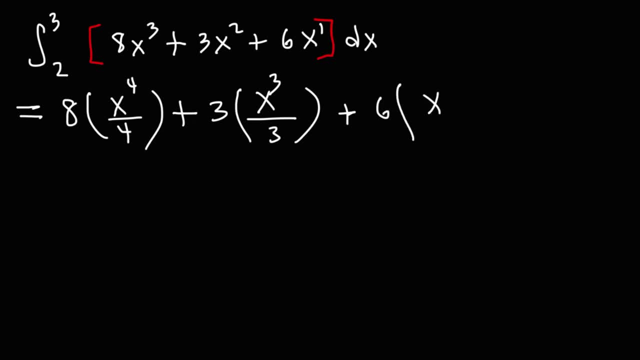 So we're going to write the constant 6, and then the variable, add 1 to the exponent. 1 plus 1 is 2, and then divide by that result. Now, as was mentioned before, because we're dealing with a definite integral, 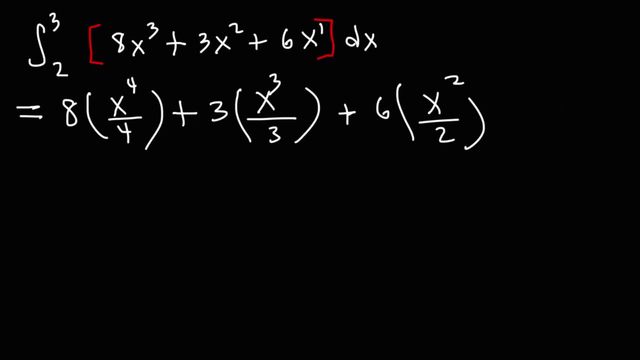 we don't need to write the constant c here, But we do need to write our limits of integration. So now let's simplify this expression: 8 divided by 4 is 2.. So we have 2.. Times x to the fourth. 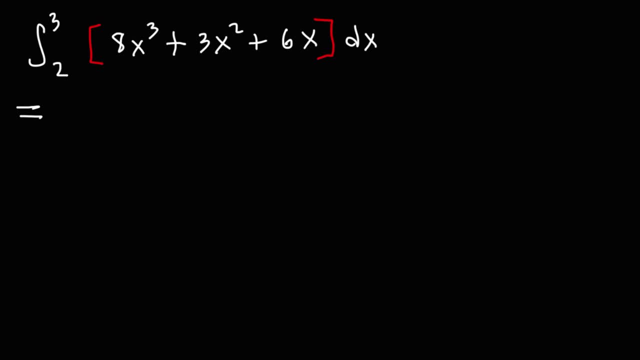 So let's say, if we want to determine the antiderivative of 4x to the seventh- So we have a constant times x to the seventh- First rewrite the constant and then find the antiderivative of x to the seventh. 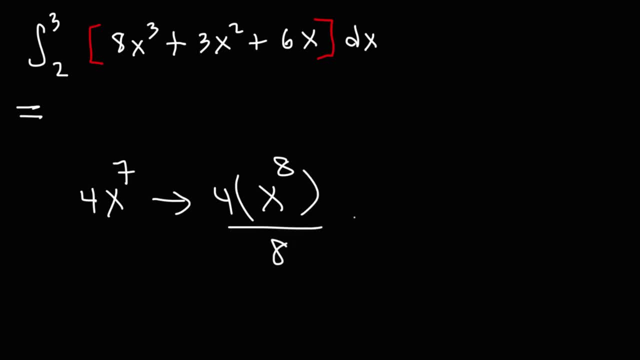 So add 1 to 7, that's 8, and then divide by that number, And after that you can reduce it. So 8 is 4 times 2.. We can cancel the 4, and so the answer is going to be x to the 8 over 2.. 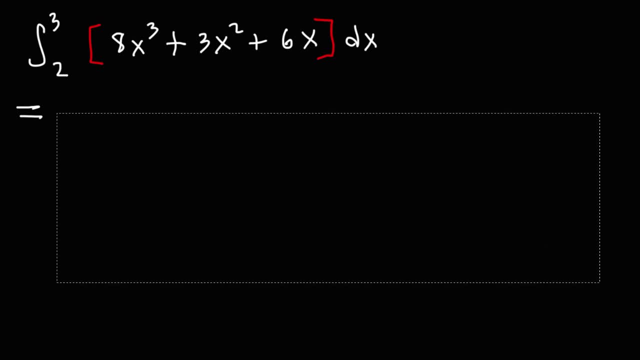 So that's how you could find the antiderivative of monomials. Now let's continue on with this example. So to find the antiderivative of 8x cubed, first we're going to rewrite the constant 8.. 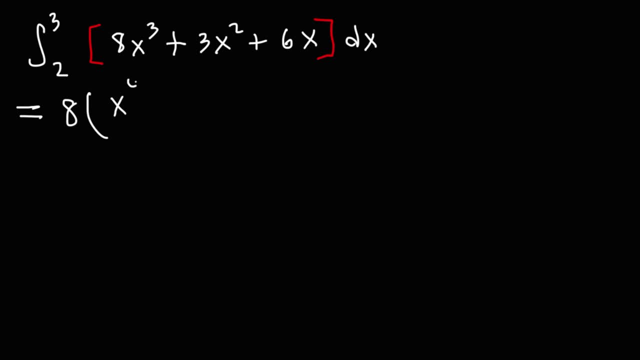 Then we're going to add 1 to the exponent. 3 plus 1 is 4.. And then we're going to divide by 4.. Now let's repeat this process for the next one. So the antiderivative of 3x squared is going to be the constant 3 times x raised to the third power, divided by 3.. 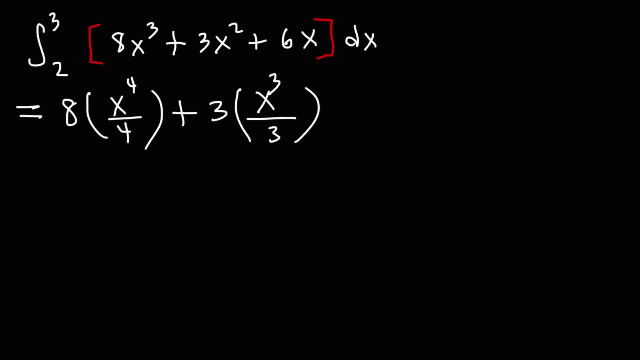 Now, what about the antiderivative of 6 times x? If you don't see a number, it's always a 1.. This is 6 times x to the first power. So, just like before, we're going to rewrite the constant. 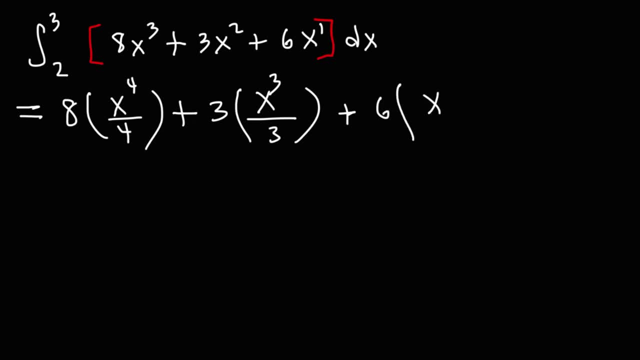 So we're going to write the constant 6, and then the variable, add 1 to the exponent. 1 plus 1 is 2, and then divide by that result. Now, as was mentioned before, because we're dealing with a definite integral, 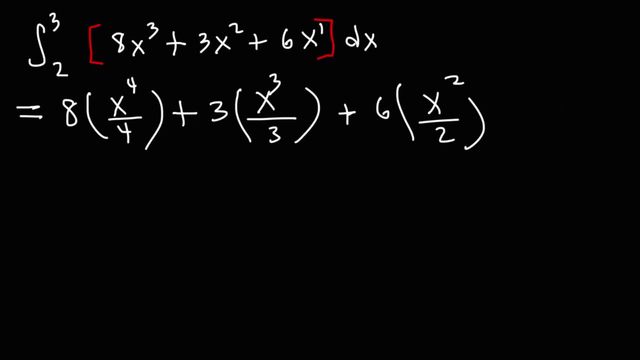 we don't need to write the constant c here, But we do need to write our limits of integration. So now let's simplify this expression: 8 divided by 4 is 2.. So we have 2.. Times x to the fourth. 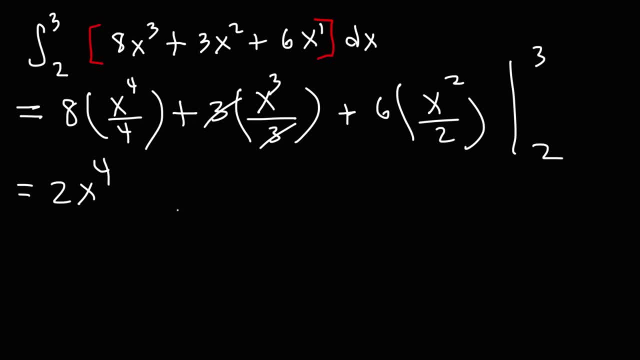 3 divided by 3 is 1.. So that cancels. So we have 1x cubed, which we can write as just x cubed. 6 divided by 2 is 3.. So then this is going to be plus 3x squared. 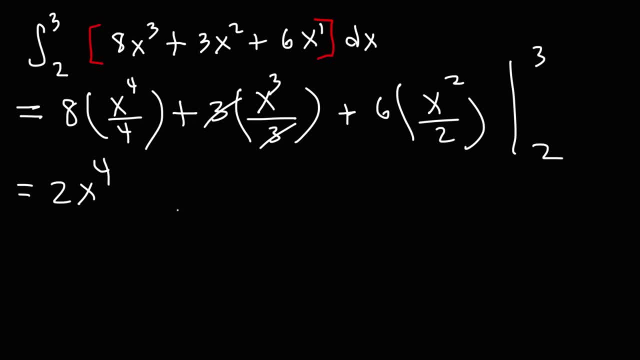 3 divided by 3 is 1.. So that cancels. So we have 1x cubed, which we can write as just x cubed. 6 divided by 2 is 3.. So then this is going to be plus 3x squared. 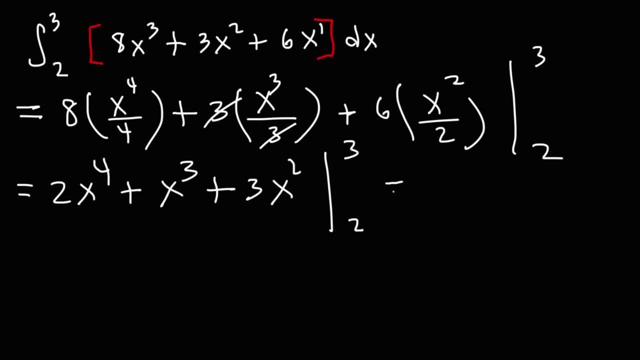 Evaluated from 2 to 3.. Now this is going to equal f of 3 minus f of 2.. And keep in mind this expression here represents lowercase f of x And this expression is the antiderivative, which represents capital F of x. 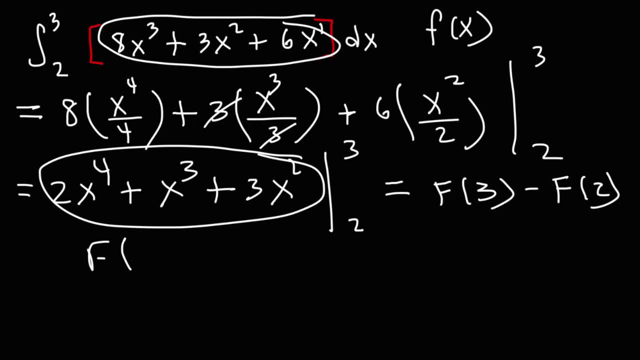 So we're going to plug in 3 and 2 into capital F of x. So in these brackets we're going to put f of 3. And here this is going to be f of 2.. So let's plug in 3 into this expression. 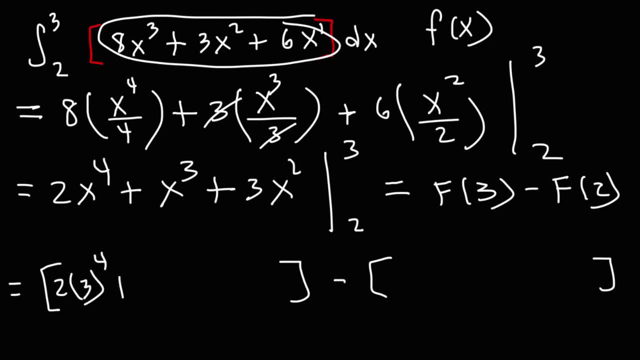 So it's going to be 2.. Times 3 raised to the fourth power Plus 3 raised to the third, power Plus 3. times 3 squared. Now, let's substitute x with 2 in the second set of brackets. 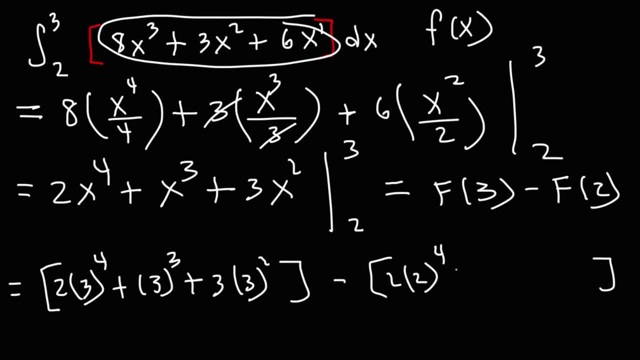 So we have 2 times 2 to the fourth power, Plus 2 to the third, Plus 3 times 2 squared. So this is f of 3.. And this is f of 2.. And this here is f of 2.. 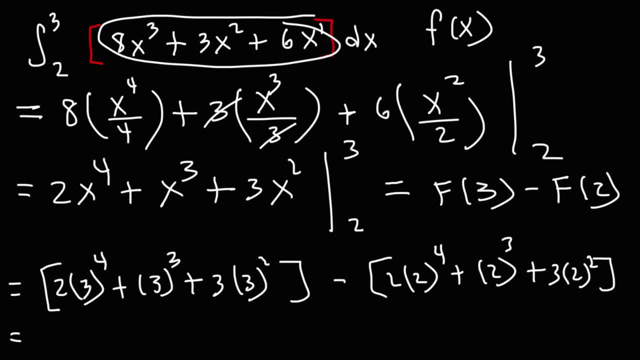 So at this point we just need to do the math. 3 to the fourth, power is 81.. And 81 times 2 is 162.. 3 to the third is 27.. 3 squared is 9.. Times 3,, that's 27 as well. 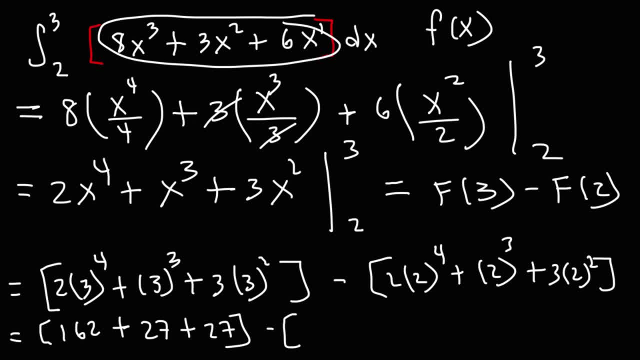 2 to the fourth power. If you multiply 4- 2s you're going to get 16.. And 16 times 2 is 32.. 2 to the third power is 8.. 2 squared is 4 times 3, that's 12.. 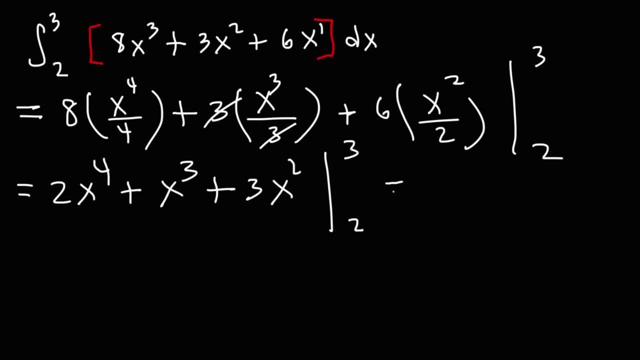 Evaluated from 2 to 3.. Now this is going to equal f of 3 minus f of 2.. And keep in mind this expression here represents lowercase f of x And this expression is the antiderivative, which represents capital F of x. 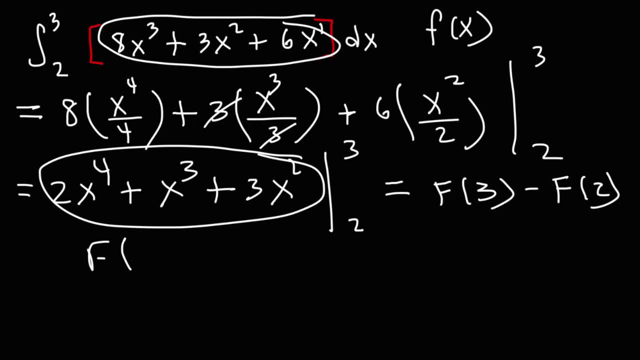 So we're going to plug in 3 and 2 into capital F of x. So in these brackets we're going to put f of 3. And here this is going to be f of 2.. So let's plug in 3 into this expression. 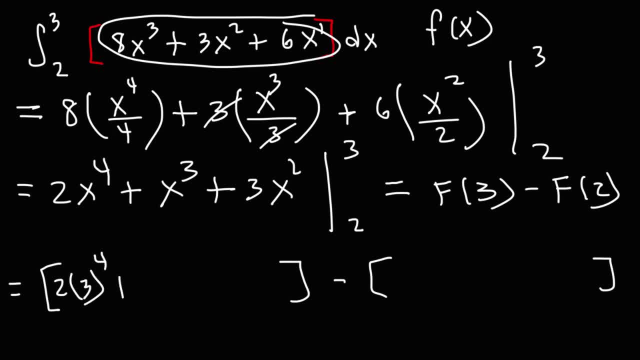 So it's going to be 2.. Times 3 raised to the fourth power, Plus 3 raised to the third power, Plus 3 times 3 squared. Now let's substitute x with 2 in the second set of brackets, So we have 2 times 2 to the fourth power. 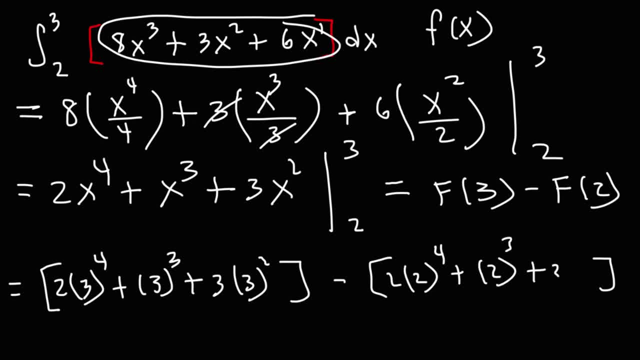 Plus 2 to the third, Plus 3 times 2 squared, So this is f of 3. And this is f of 3. And this here is f of 2.. So at this point we just need to do the math. 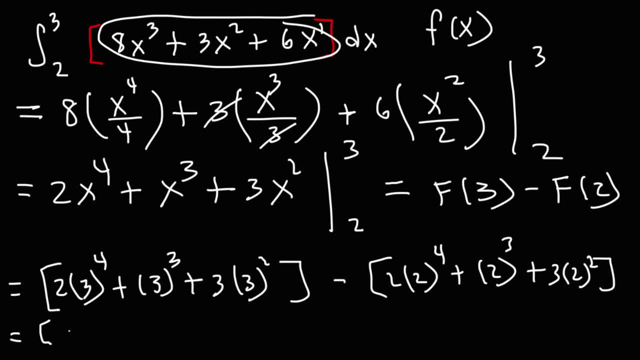 3 to the fourth power is 81.. And 81 times 2 is 162.. 3 to the third is 27.. 3 squared is 9.. Times 3, that's 27 as well. 2 to the fourth power. 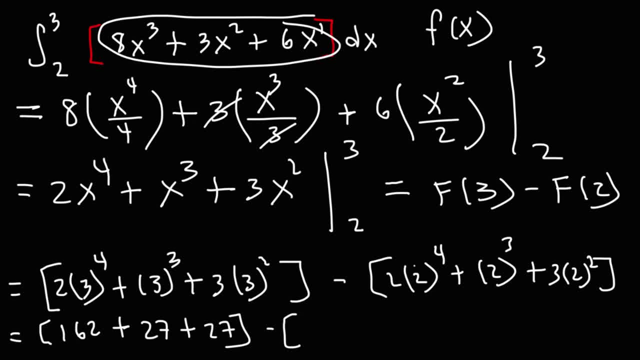 If you multiply 4 2's, you're going to get 16.. And 16 times 2 is 32.. 2 to the third power is 8.. 2 squared is 4.. Times 3,, that's 12.. 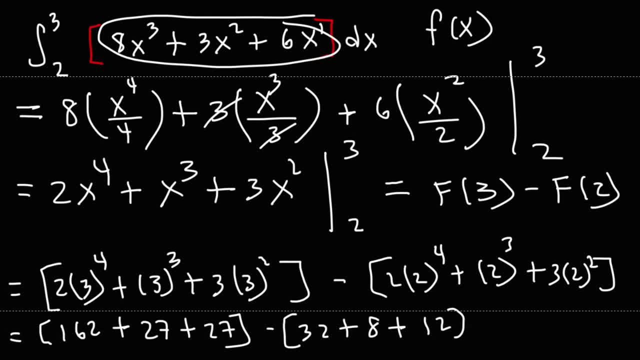 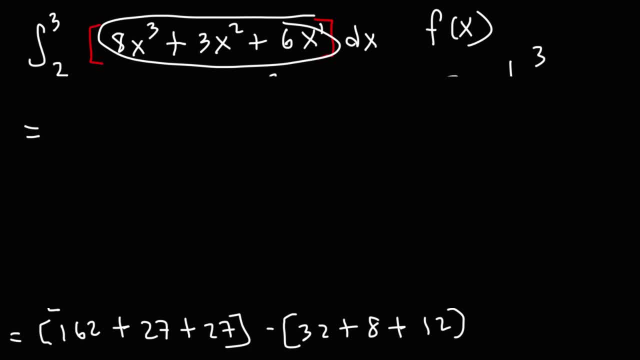 2 to the fourth, power is 12.. 27 plus 27.. We no longer need the brackets anymore. 27 plus 27 is 54.. 32 plus 8 is 40. And 40 plus 12 is 52.. 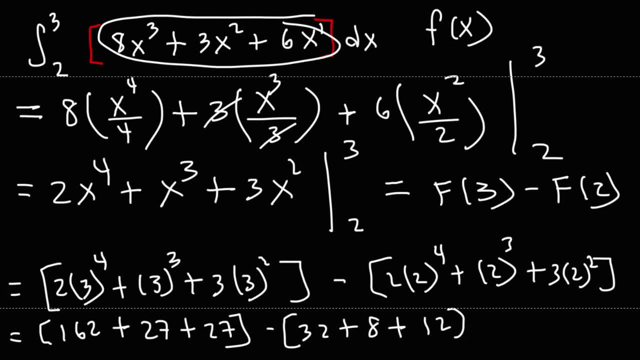 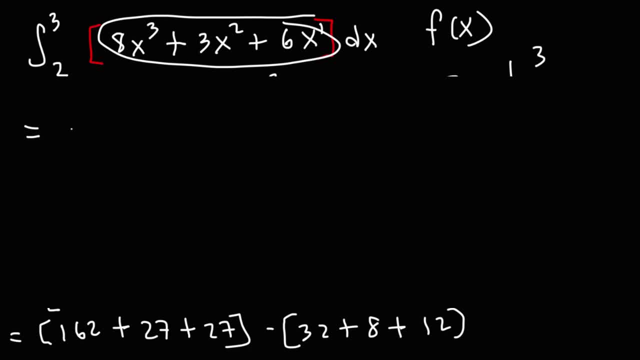 So I'm going to subtract the 12.. 27 plus 27.. We no longer need the brackets anymore. 27 plus 27 is 54.. 32 plus 8 is 40. And 40 plus 12 is 52..